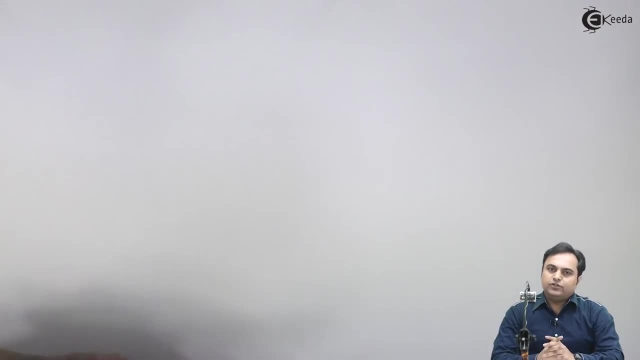 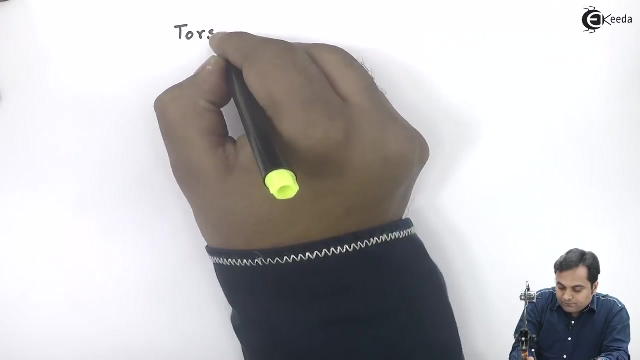 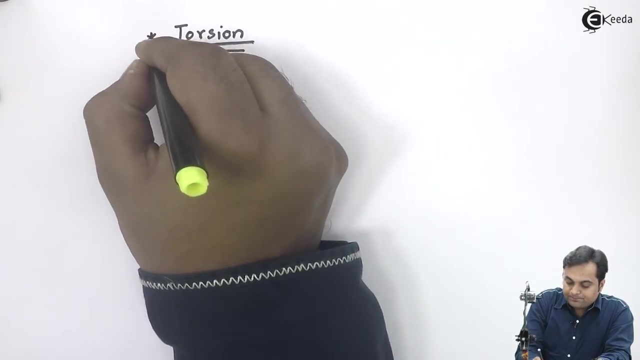 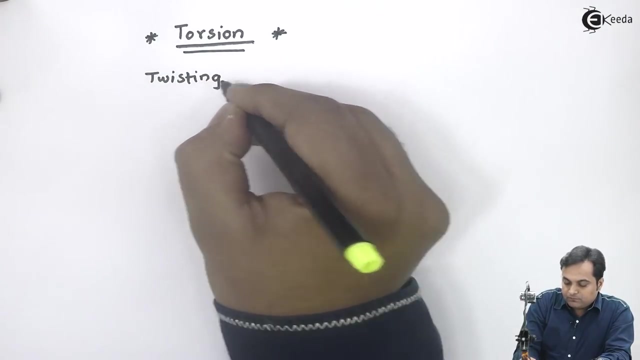 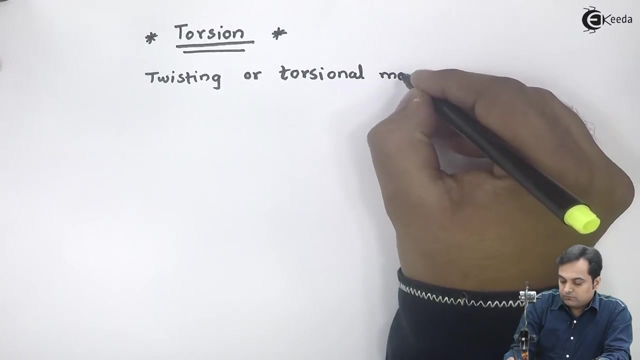 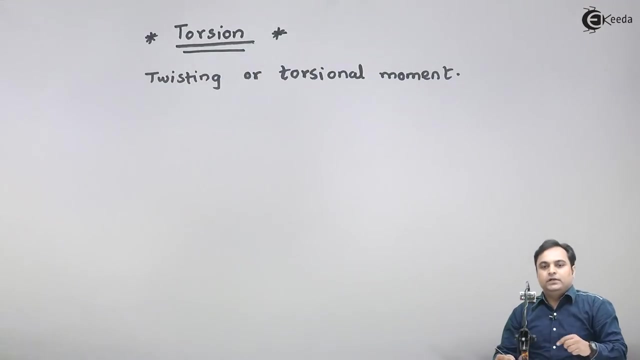 Hello students, let us start with a new topic today in SOM, The name of the chapter is Torsion. When we say torsion, the meaning of torsion is twisting or torsional moment. So whenever we talk about torsion it is such that we have a twisting or you can say, torsional moment. 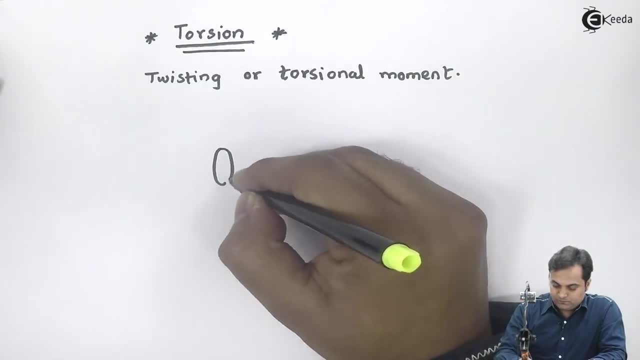 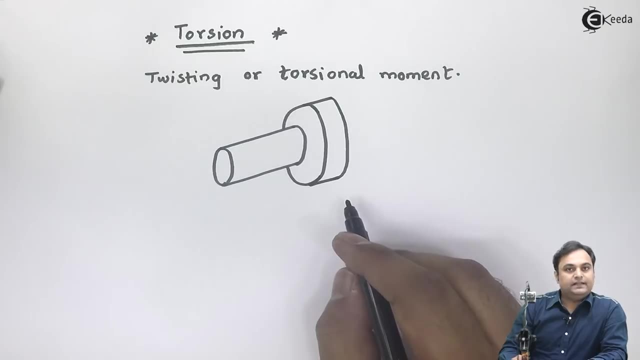 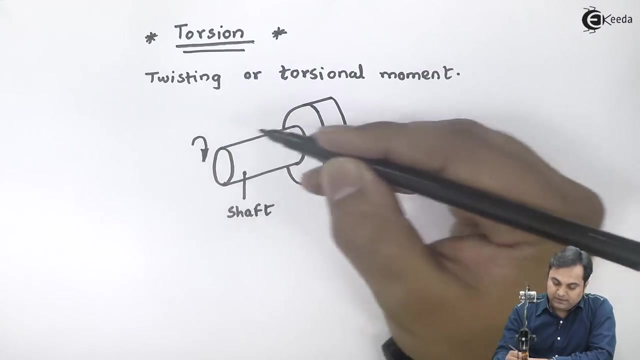 This can be explained with a diagram. Here we have a diagram in which there is a shaft and here we have a bearing. Shaft is that member which rotates. So if we are rotating the shaft and it is supported inside a bearing, if a shaft rotates in clockwise direction, 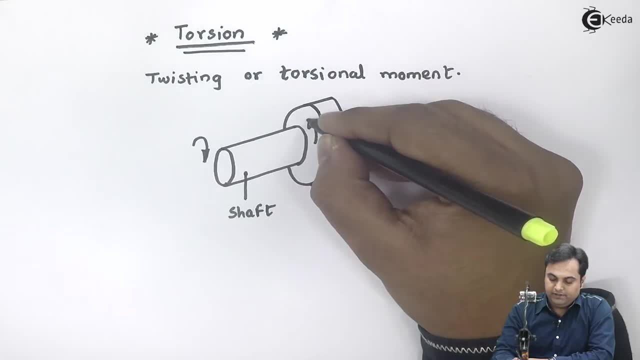 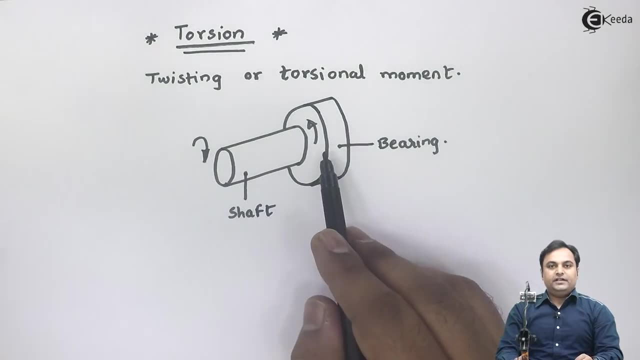 bearing will try to oppose its motion in the opposite direction. So here at the shaft we are having clockwise rotation, At the bearing end we are having anticlockwise rotation. Because of these two unequal torques there is twisting of this shaft. 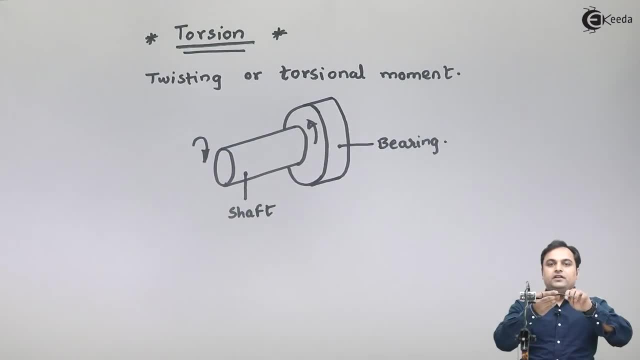 This example is like if I have this pen, if I am rotating the pen in two opposite directions at the each of the ends, if I rotate it in the opposite direction, then this would be: this pen would be twisting, and that twisting is nothing but torsion. 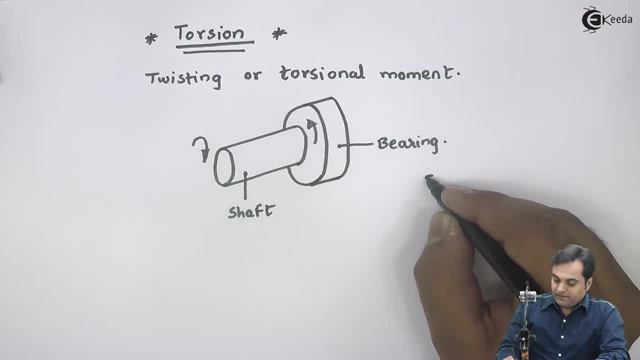 Now, when we say torsion, torsion can also be called as torque. Torsion can also be called as torque. And torque is the product of tangential force- Ft- multiplied by the radius of the shaft. And torque is the product of tangential force- Ft- multiplied by the radius of the shaft. 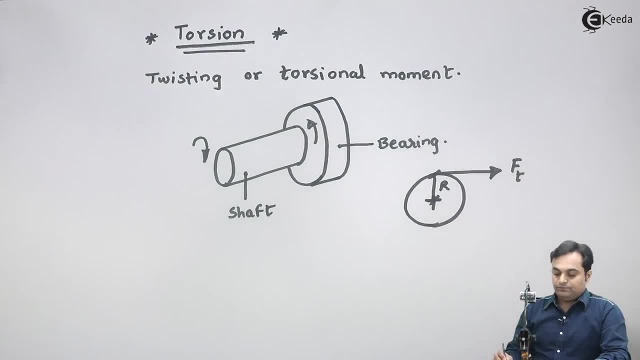 Because of the product of Ft into R, this shaft would be rotating. So I can say that torque T is equal to tangential force into radius of the shaft. The unit is tangential. force would be in Newton, radius would be in mm. 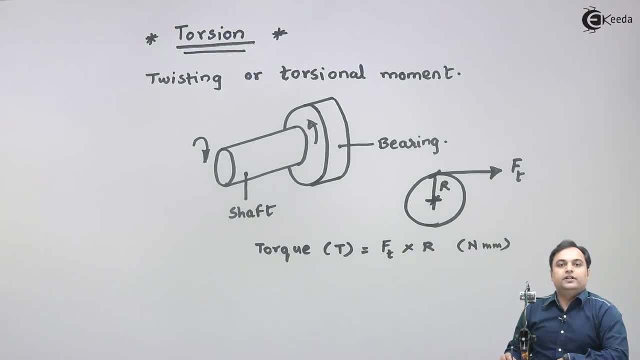 So here I have the torque in terms of Newton mm. So, in other words, whenever we talk about torsion, the simplest way to understand torsion is that it is twisting, and twisting is produced by two unequal moments: One which would be in clockwise direction and the other in anticlockwise direction. 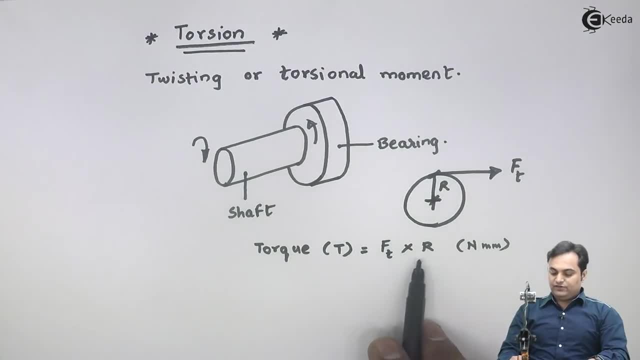 Simply, we can give torque as tangential force into the radius of the shaft. That is, this product gives a rotation and it would be in the direction of Ft. So here I have clockwise rotation. So this was a brief concept regarding torsion. 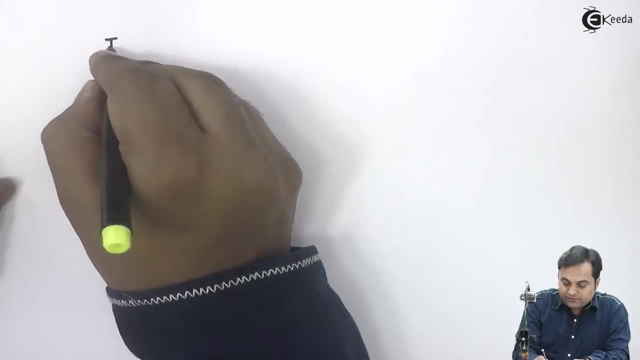 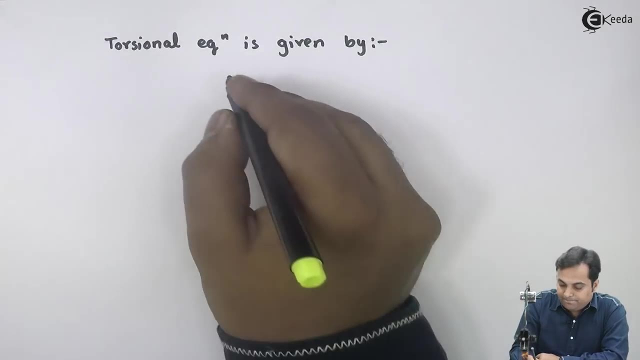 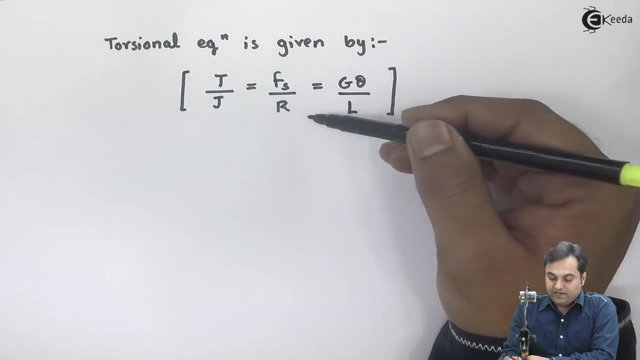 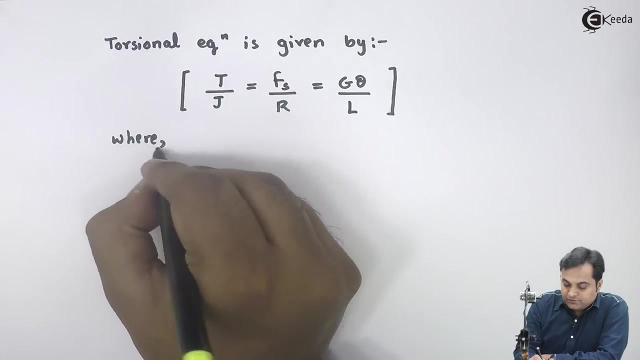 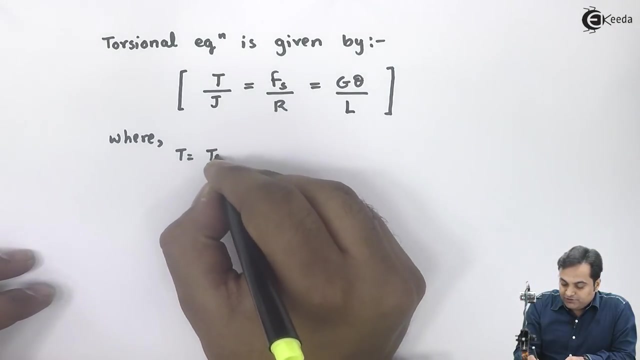 Now let me give you the torsional equation. The torsional equation is given by T, by J is equal to Fs, by R is equal to G theta, by L. Here I will be defining all the terms. T is the torque, or twisting moment. 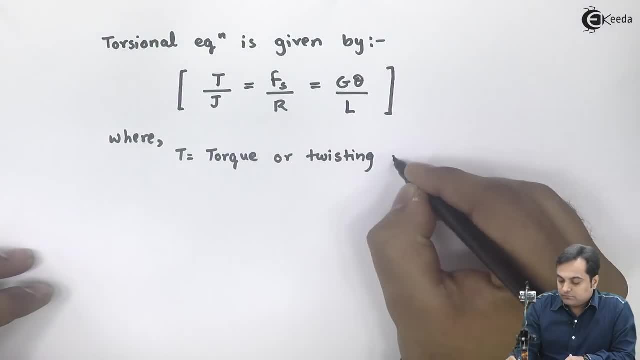 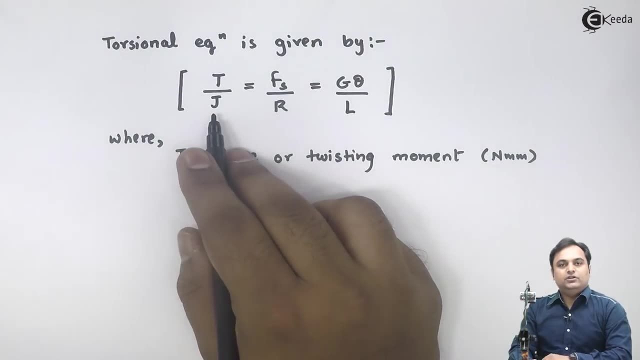 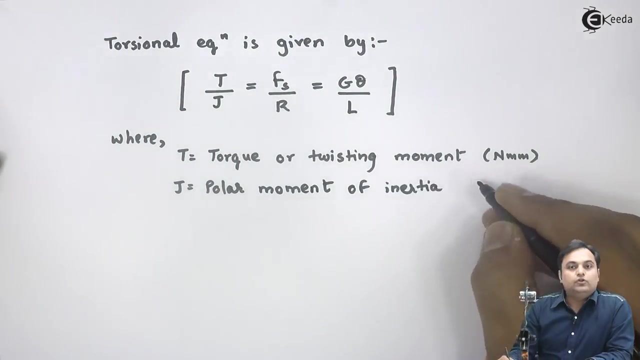 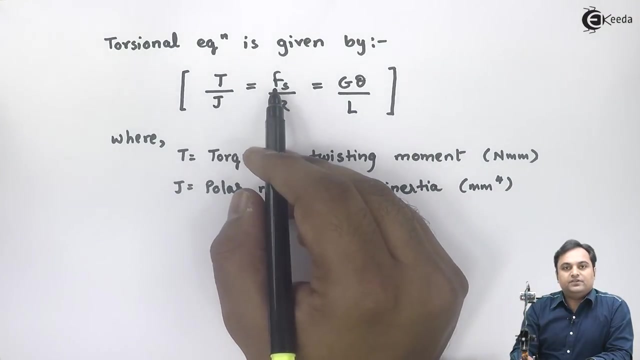 T is the torsional force. T is the torsional force. T is the torsional force. Unit will be in Newton mm. J is called as polar moment of inertia. Unit will be in mm raised to 4. Fs would be called as shear stress. 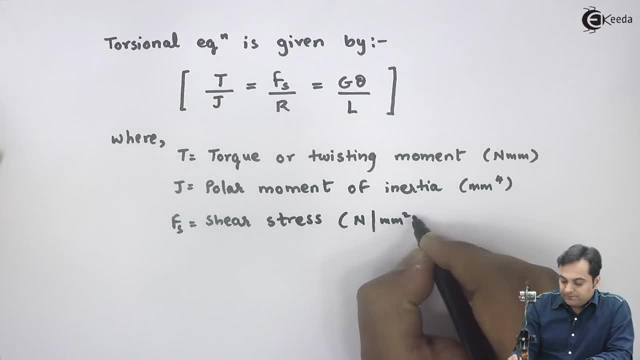 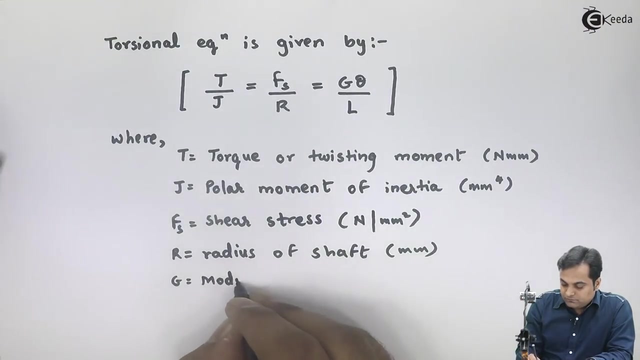 Unit will be Newton per mm square. fez will be comfortable. Capital R will be the radius of shaft. capital R will be the radius of shaft. G means modulus of rigidity. Unit will be Newton per mm square. Unit will be Newton per mm square. 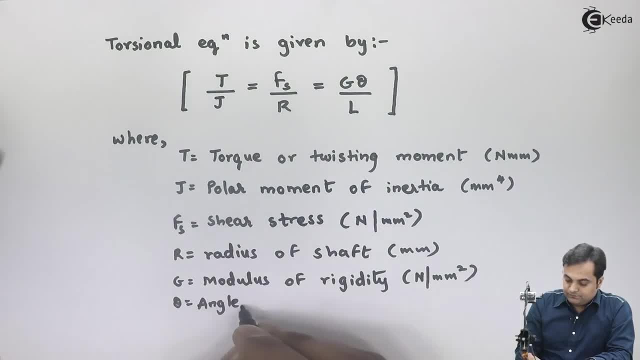 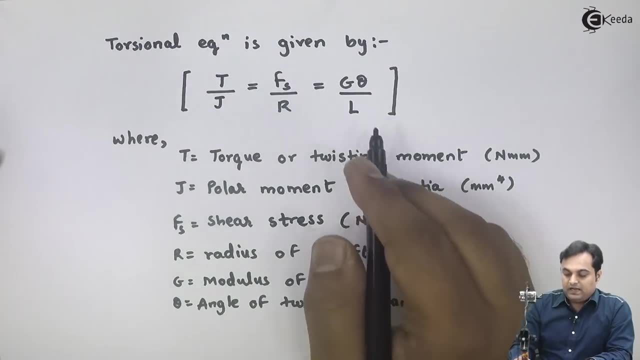 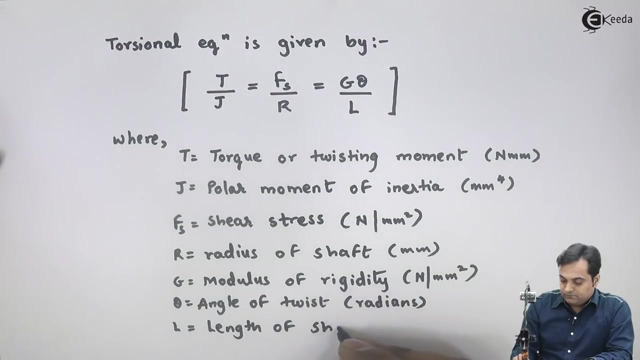 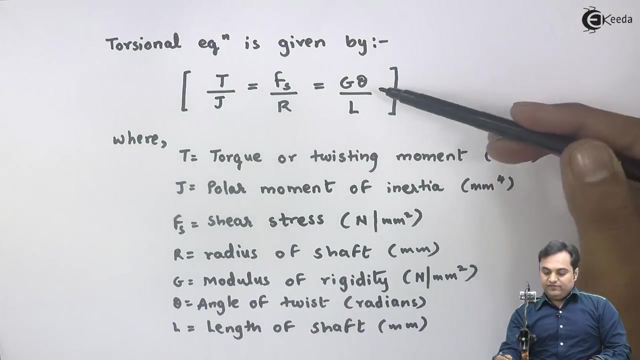 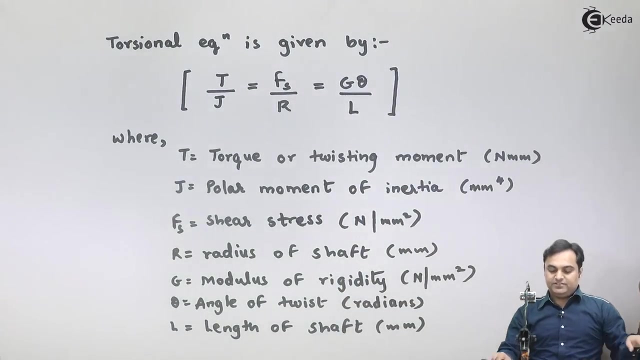 Theta is angle of twist. Theta is angle of twist will be radians and capital L it indicates the length of shaft, which will be in terms of mm. so this is the torsional equation which we have, and here I have defined all the terms. now, this angle of twist, it can be explained in such a way that, if we have this diagram, 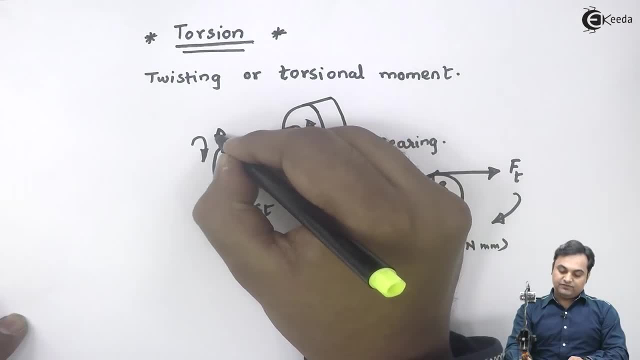 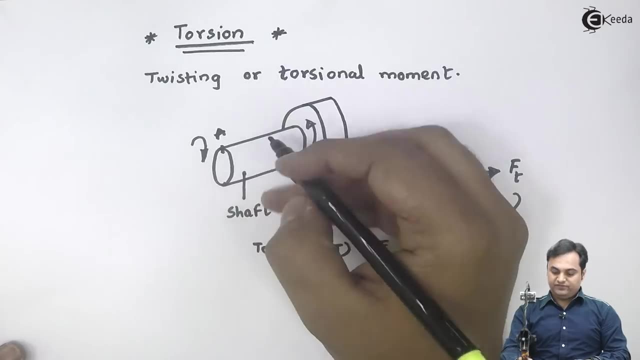 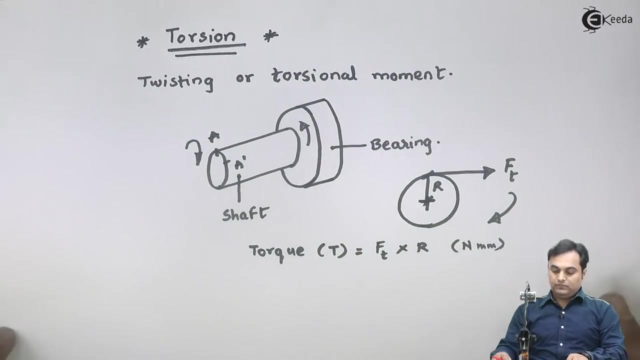 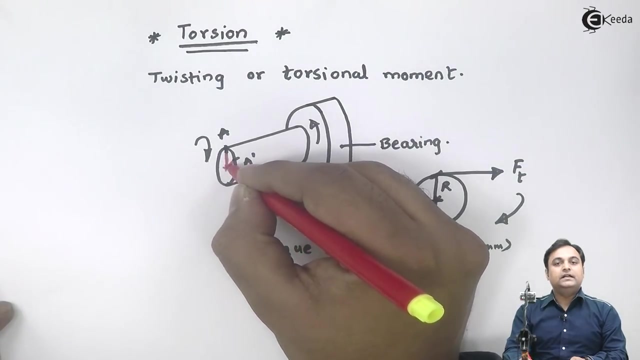 of a shaft. I consider point A on the shaft and when the twisting occurs, this point A will be shifted to another location called as A' and from the centre of the shaft. if I consider this here, I have a small angle, and this small angle would be called as theta. 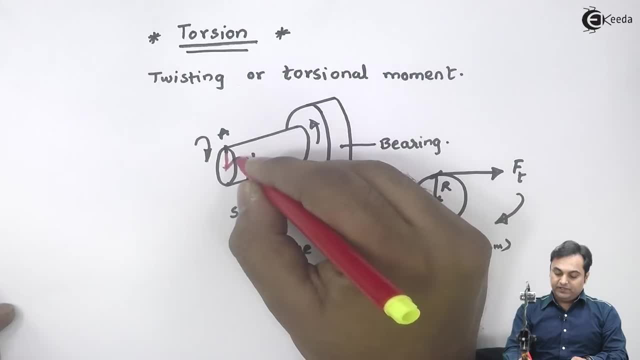 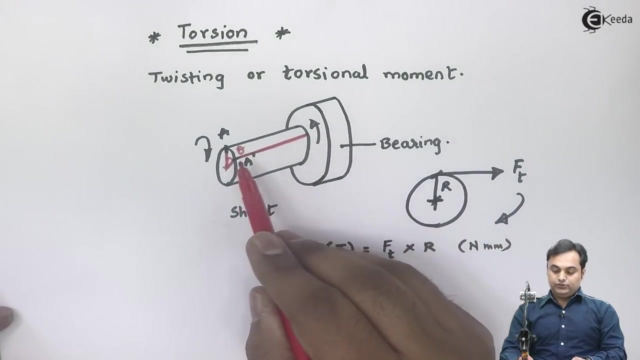 that is the angle of twist, And this angle would be called as theta, And this angle of twist would be there all along the length of the shaft. So here I have theta, which is the angle of twist, which would be constant along the length. so this is angle of twist, theta. 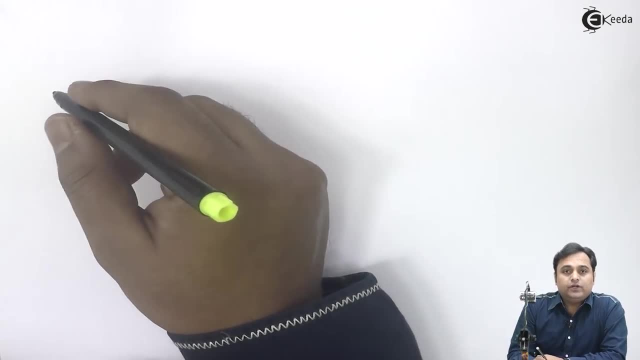 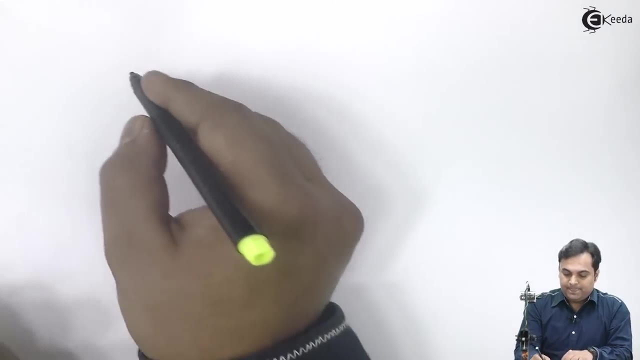 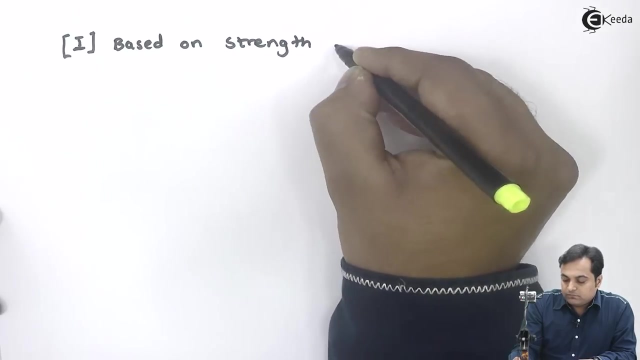 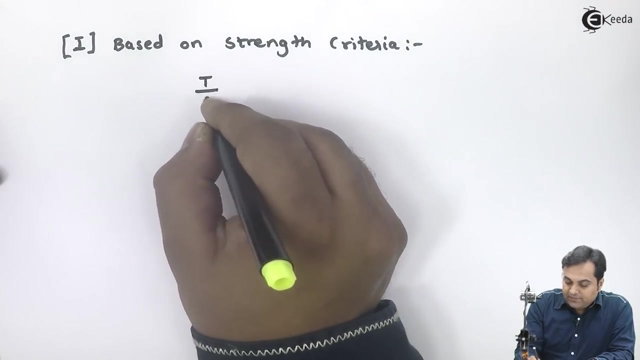 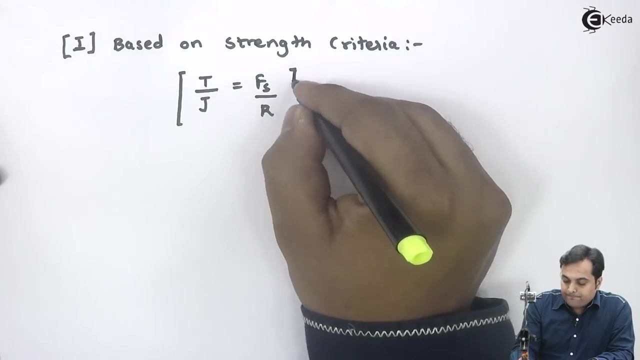 Next, let me give you all two equations to solve the problems on torsion. the first equation would be called as based on strength criteria. So, based on strength criteria, we have the torsional equation as T by J is equal to Fs by R. this is called a strength criteria because here we have shear stress. 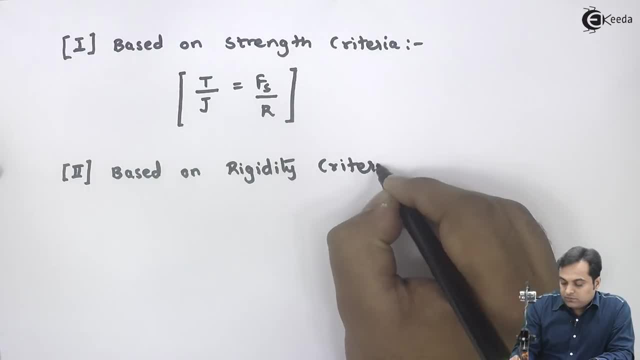 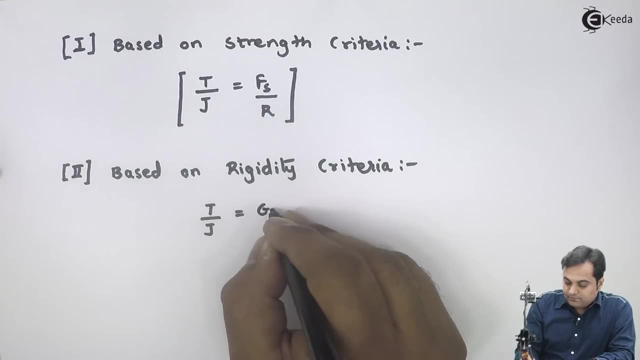 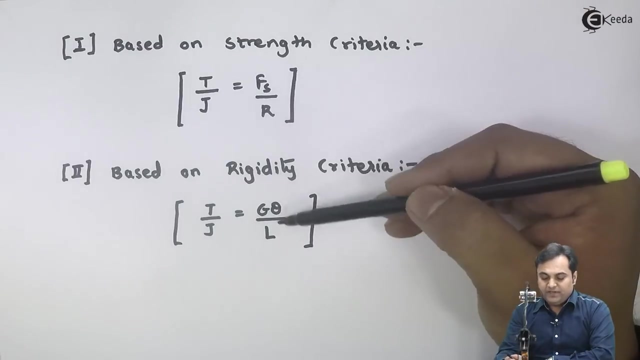 next, based on rigidity criteria I have the formula: T by J is equal to G, theta by L. this is called as rigidity criteria, because here I have modulus of rigidity, G and angle of twist, theta. so based on these two criteria we can solve any problem related to shafts.